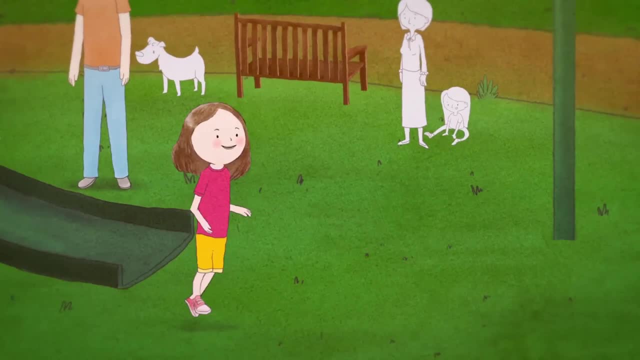 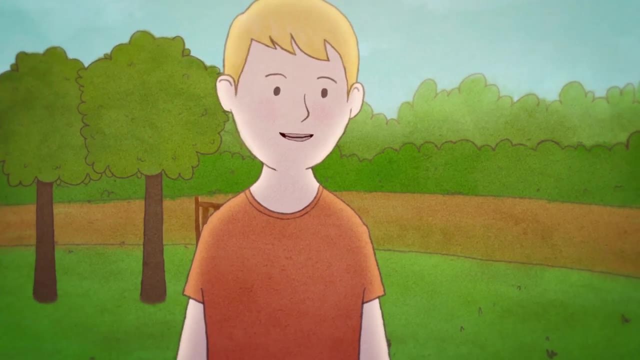 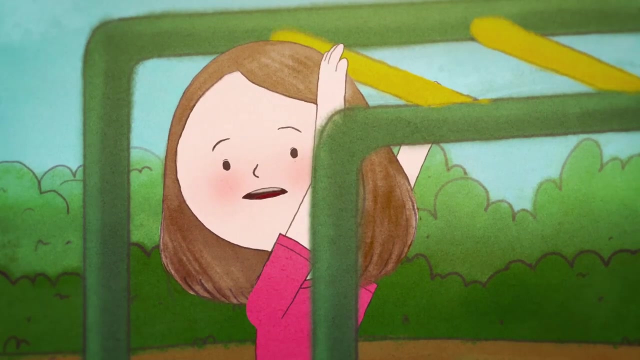 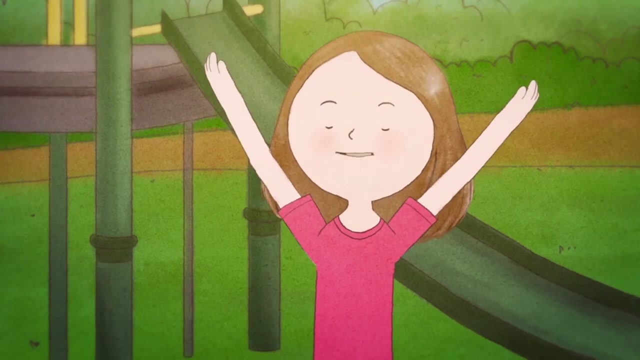 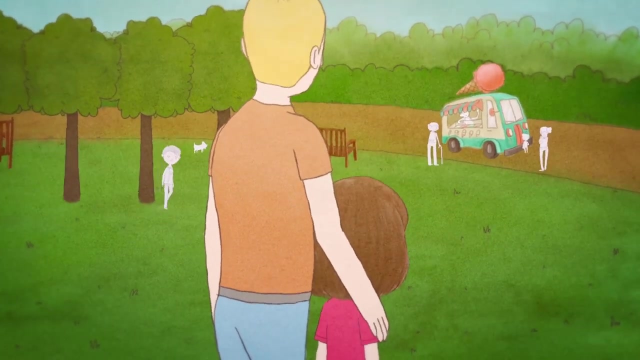 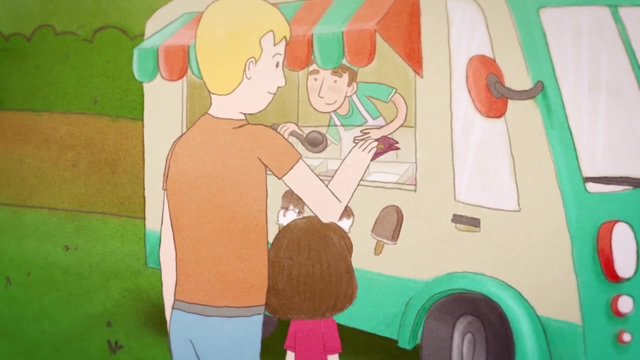 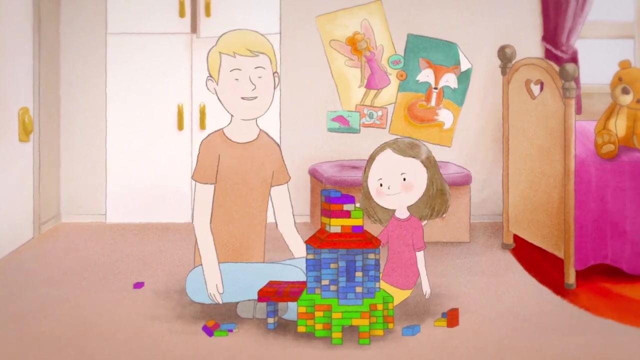 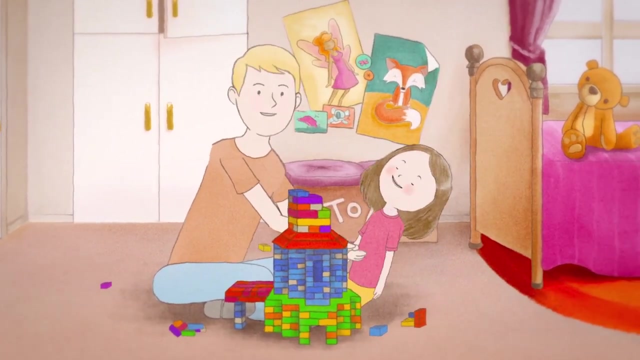 Here I can help you. Would you like an ice cream, Anna? I love ice cream, but Mum hardly ever lets me have it. Oh, don't worry, we can make it our little secret. Hey, I know a really great game. that's lots of fun. 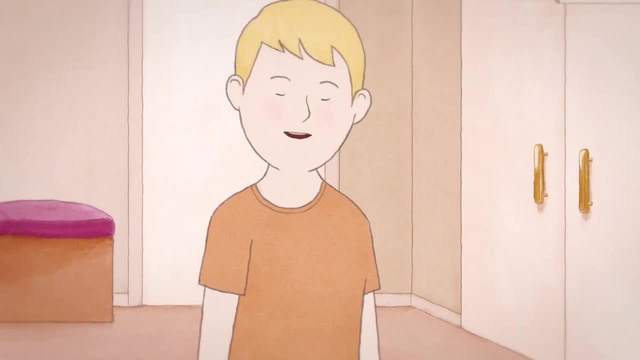 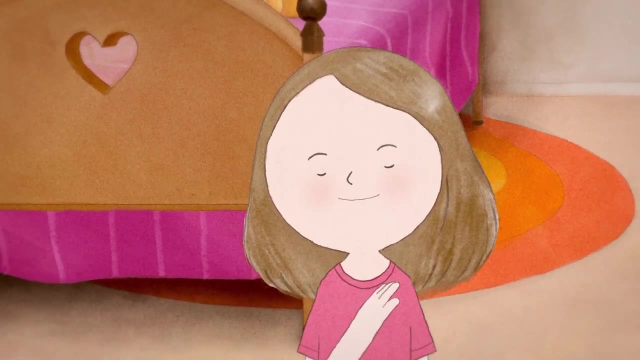 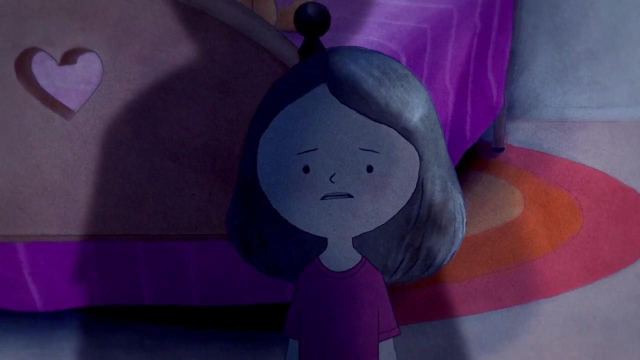 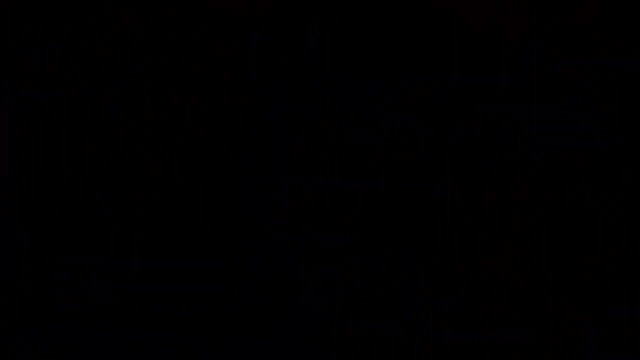 Can we play it? Well, it's a secret, just like the ice cream. Can you keep a secret? Yes, I promise I won't tell anyone. I don't want to tell anyone. So tell me, What kind of game is this? What are you doing? 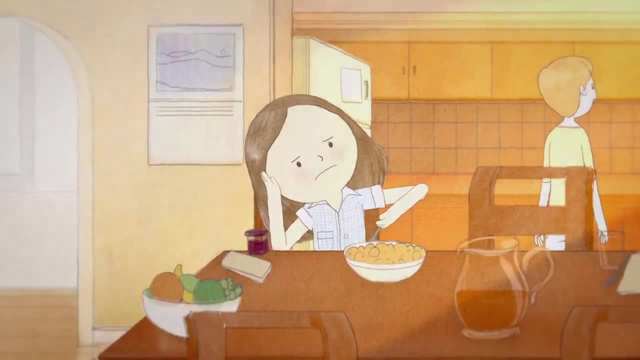 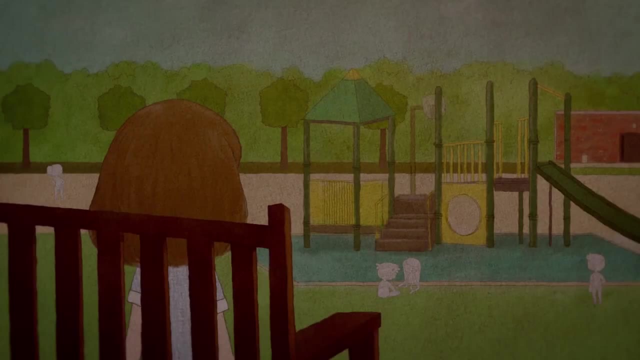 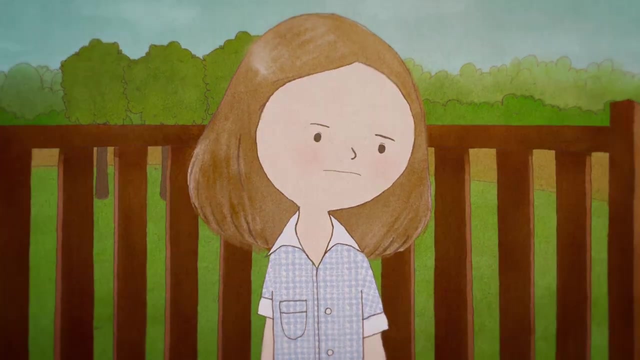 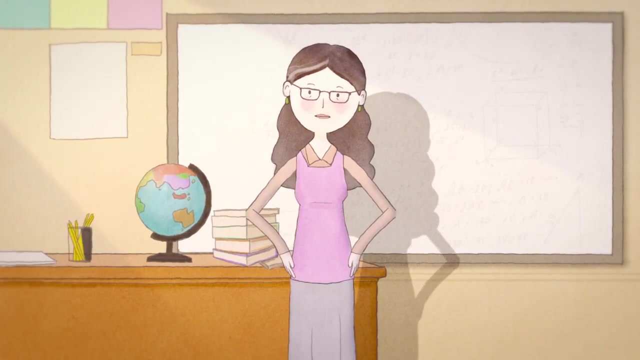 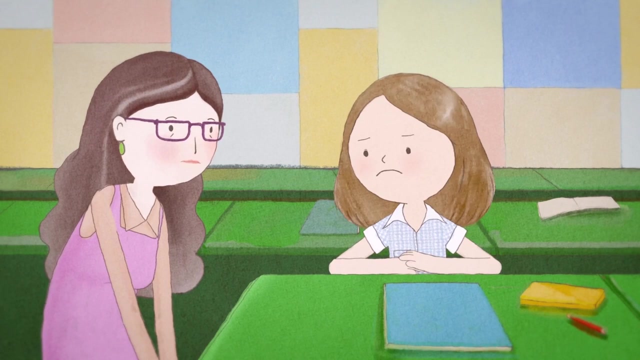 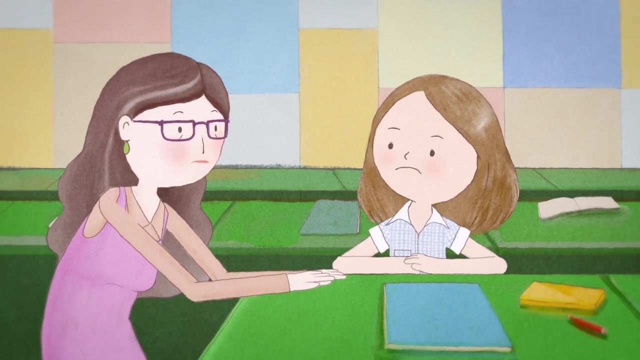 What kind of game is this? What are you doing, Anna? Anna, I asked you a question and it. can you please stay back a moment. you don't seem like yourself, Anna. is everything okay? something bad happened, but I'm not allowed to tell anyone. if you have a secret that is making you. 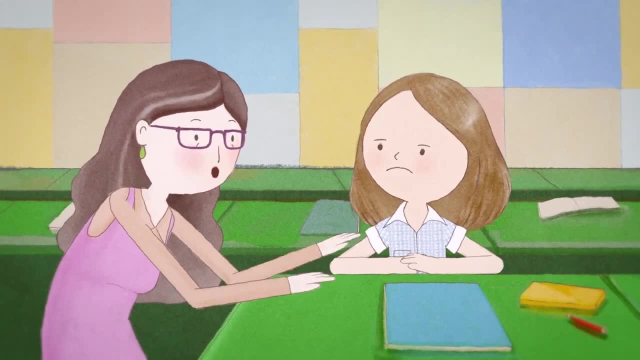 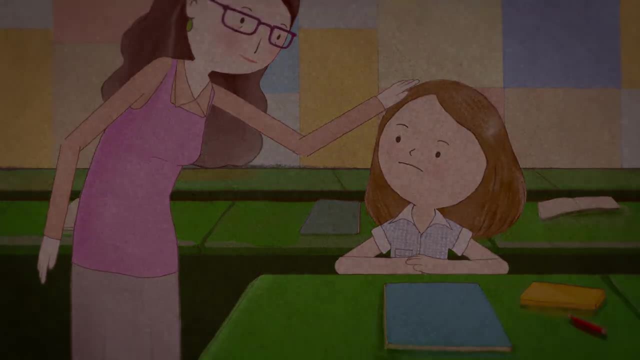 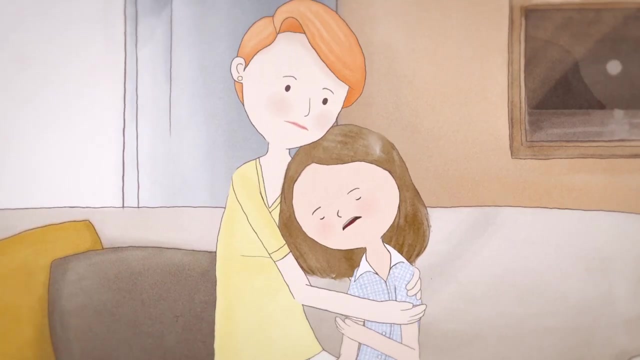 upset. it's very important to tell an adult you trust so that we can help you and make you feel better. I'm going to call your mum and dad to come and pick you up. okay, Anna, you really need to tell me what's upsetting you, but it's. 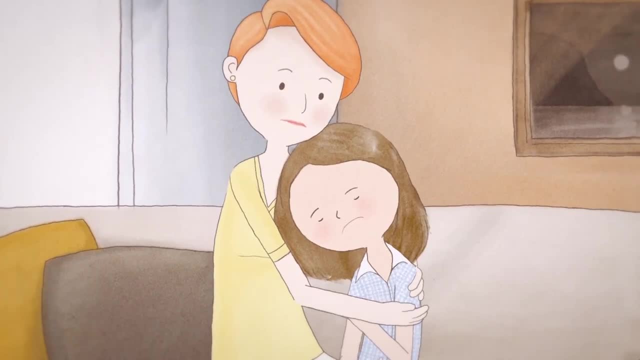 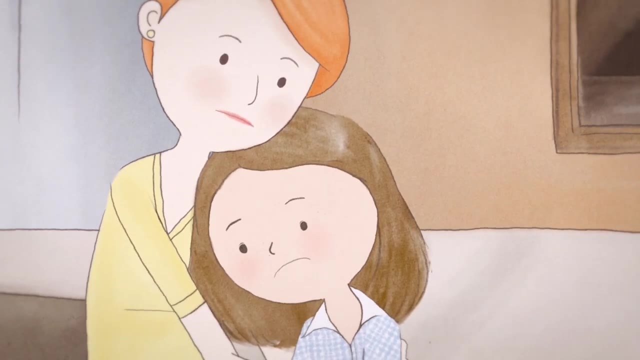 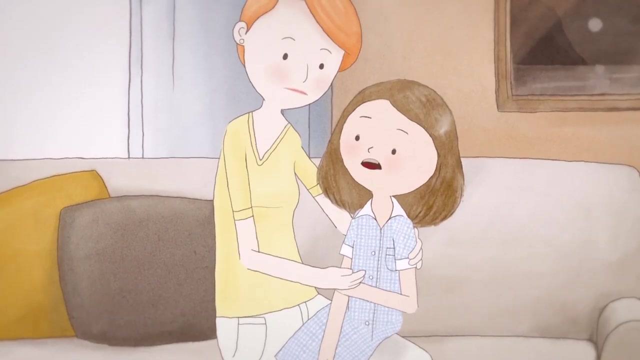 something bad and you and dad will be very angry with me. I promise we won't get cross. I love you and there is nothing that you cannot tell me. well, when Mike was looking after me, we- um he, he made me play a game of. I didn't like what happened in this game. Mike touched me in my private parts. I.